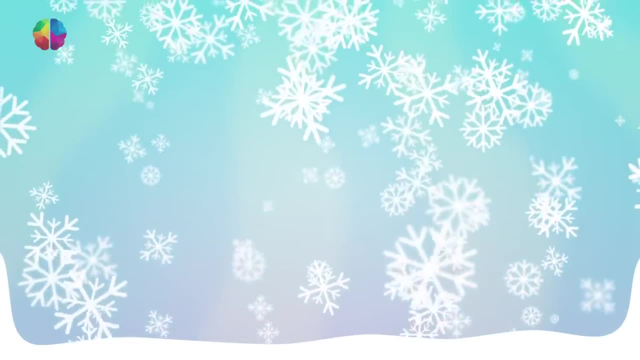 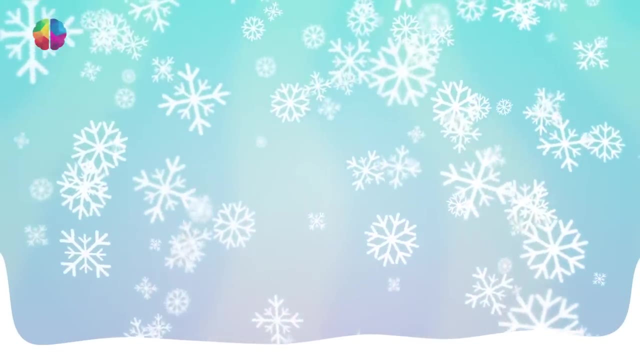 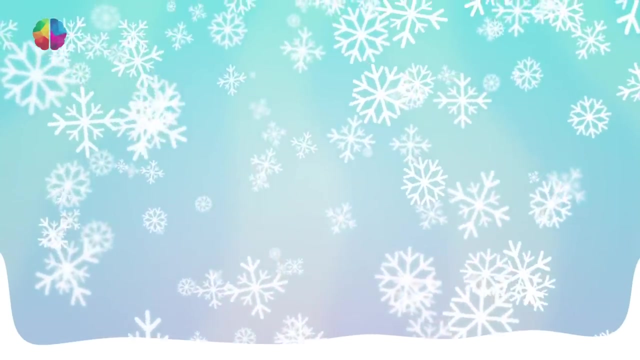 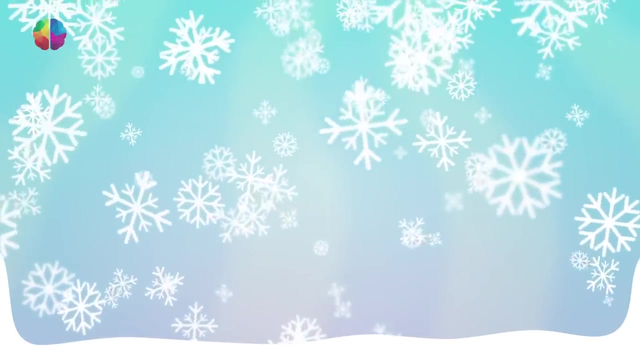 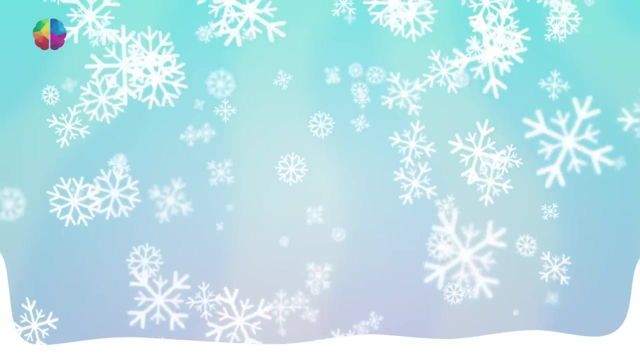 Embrace the cold sensations all over your skin. This icy feeling gets deeper and deeper. You can feel the cold air all over your skin. This icy feeling gets deeper and now even the core of your body is cold. Slowly lower yourself to the ground and lie on the floor. 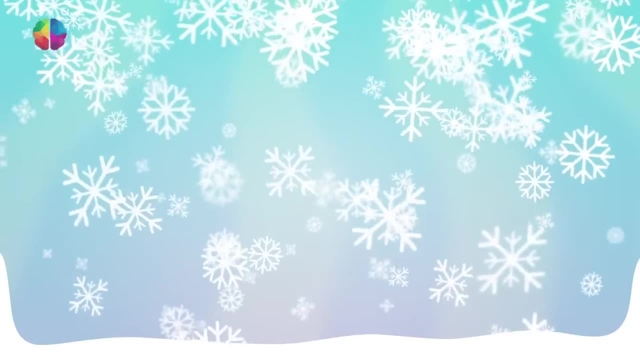 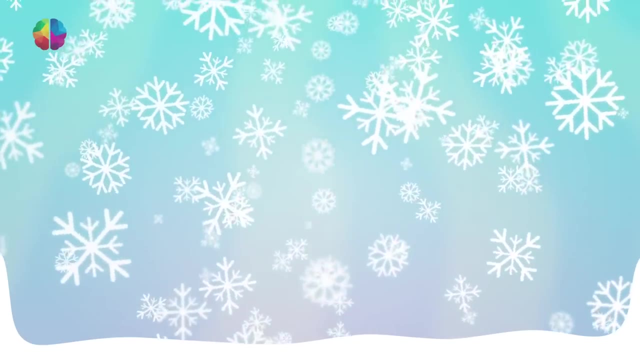 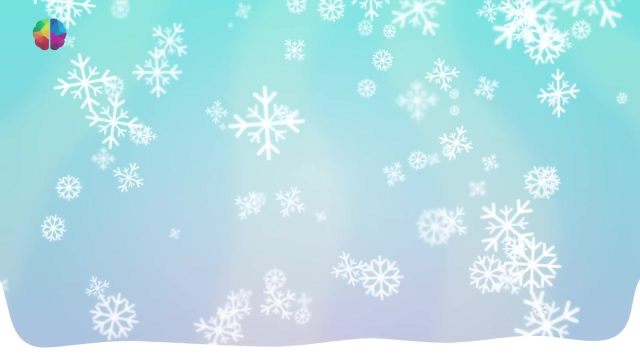 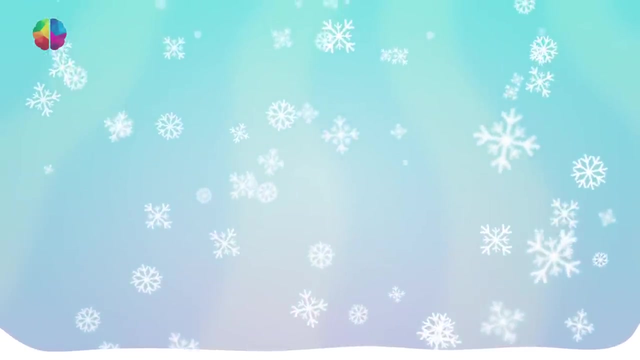 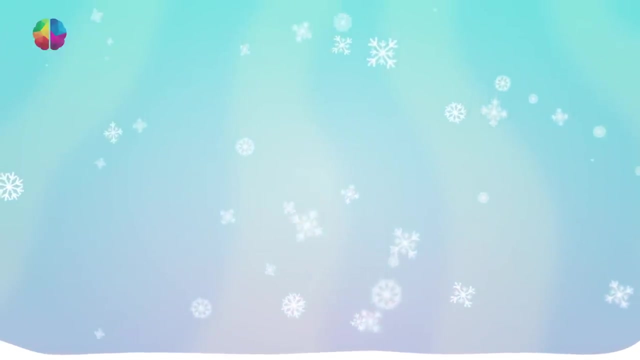 Slowly lower yourself to the ground and lie on the floor. Now close your eyes. Imagine the snow that's covering you is melting, And as it does so, let your muscles relax too. Your back slowly relaxes. Your shoulders melt towards the ground. 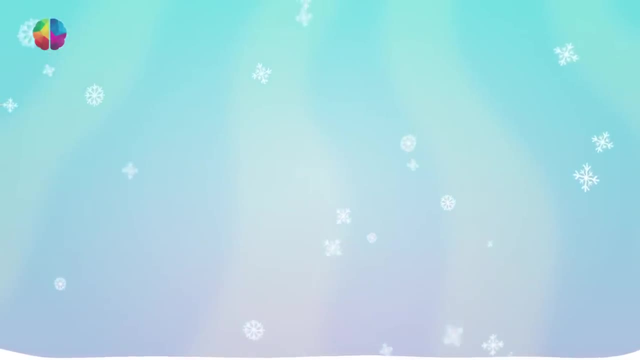 Your shoulders melt towards the ground And the muscles in your arms melt and drip onto the floor. And the muscles in your arms melt and drip onto the floor. Just lie there for a few more moments and enjoy this relaxation. Just lie there for a few more moments and enjoy this relaxation. 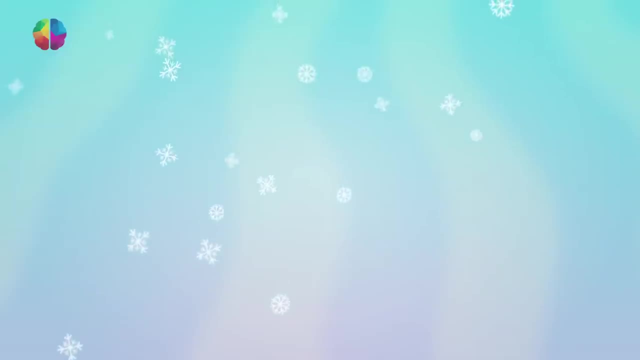 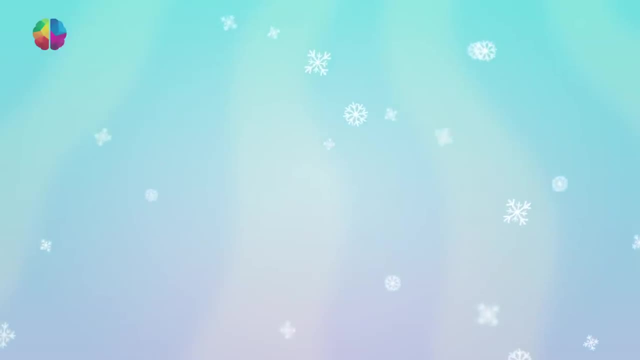 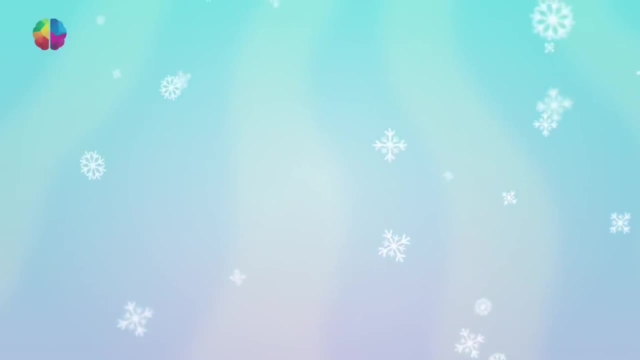 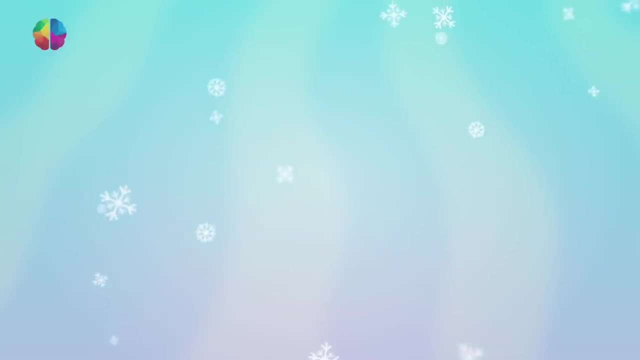 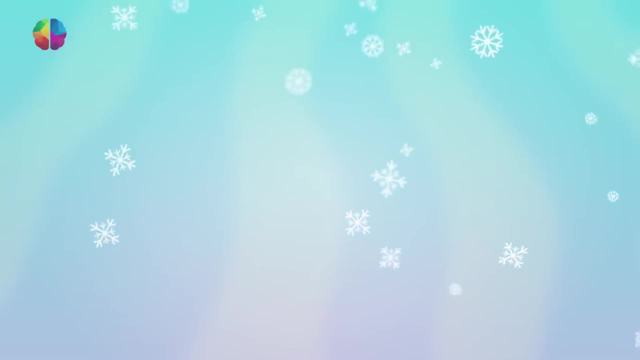 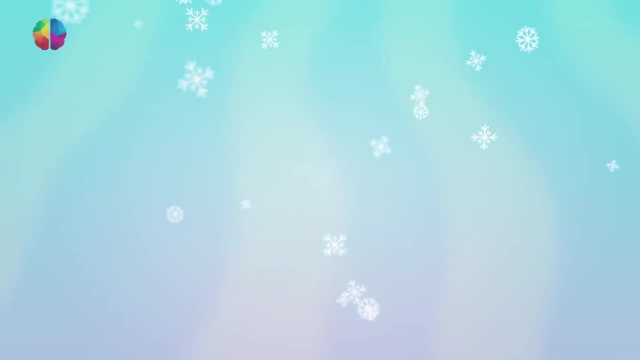 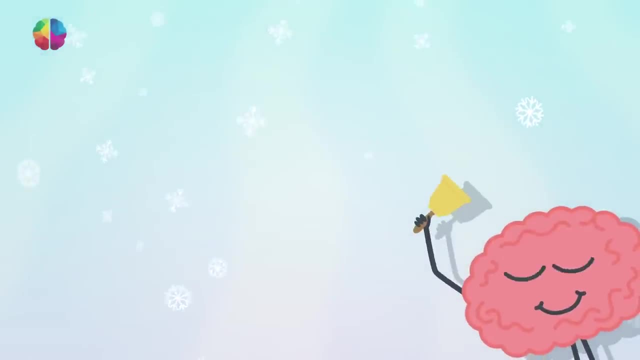 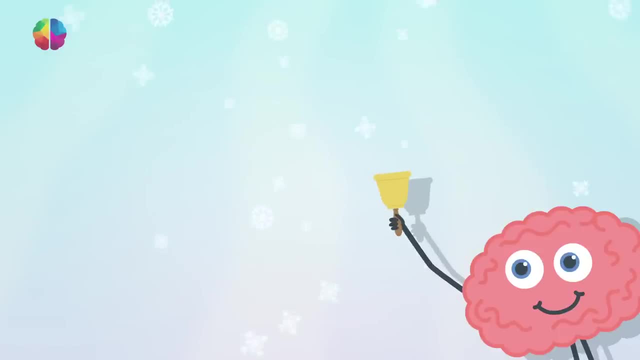